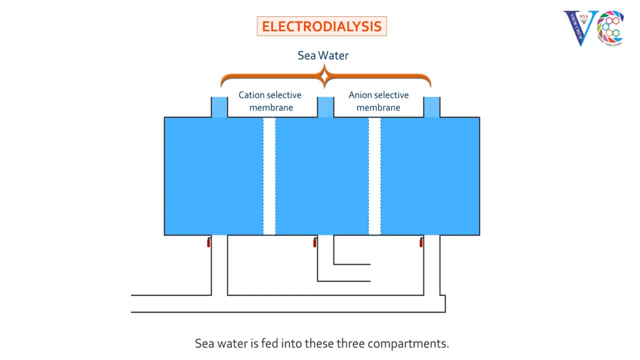 The contents of the container. The contents of the container, The contents of water that has been treated, are aged forズ نے 13 days. The application of electro-dialysis is the practically reactivation of And thente that is entered in the container. There are two added compartments in total. They might have different cables or faculties necessary As such. the interpreting of the components and its equivalent links to the entire fast mode movement of ions, The dis senators, the changes of electrode compartments and electrons and electrons. 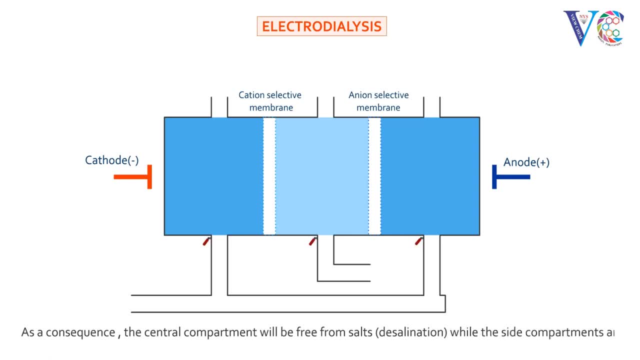 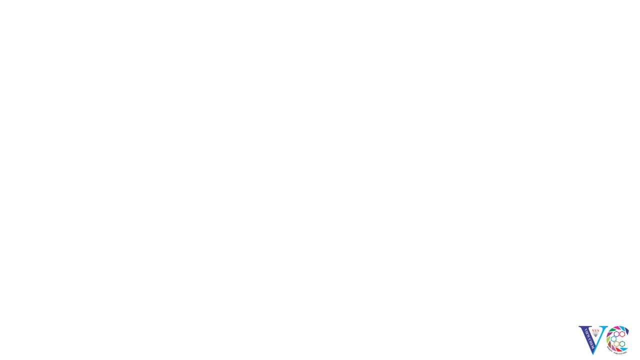 from salts. that is desalination, while the side compartments are concentrated with salty water, Salt-free water and saline water will be drawn out separately. Advantages: It is an economical method. It can be carried out at room temperature. It is a continuous process. 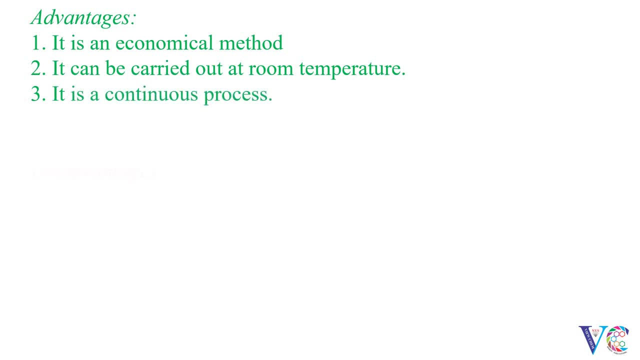 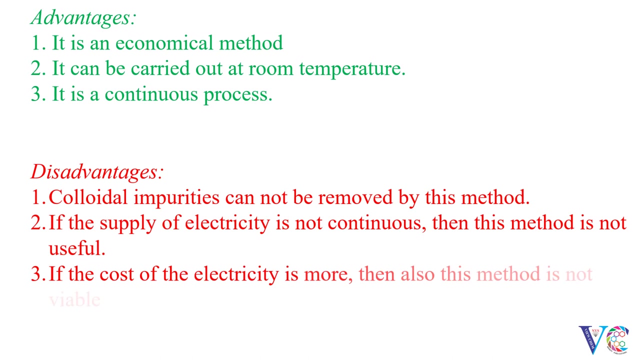 Disadvantages: Colloidal impurities cannot be removed by this method. If the supply of electricity is not continuous, then this method is not useful. If the cost of the electricity is more, then also this method is not viable. Osmosis. 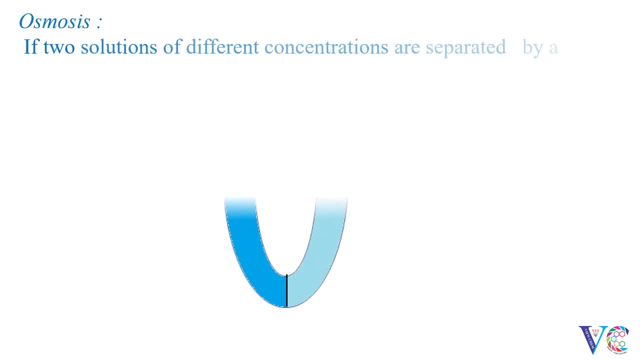 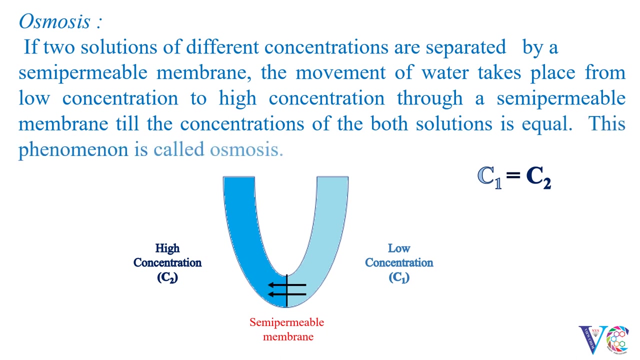 If two solutions of different concentrations are separated by a semi-permeable membrane, the movement of water takes place from low concentration to high concentration through a semi-permeable membrane till the concentrations of the both solutions are equal. This phenomenon is called osmosis. 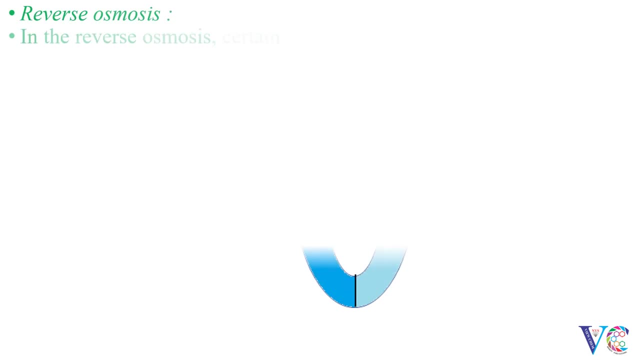 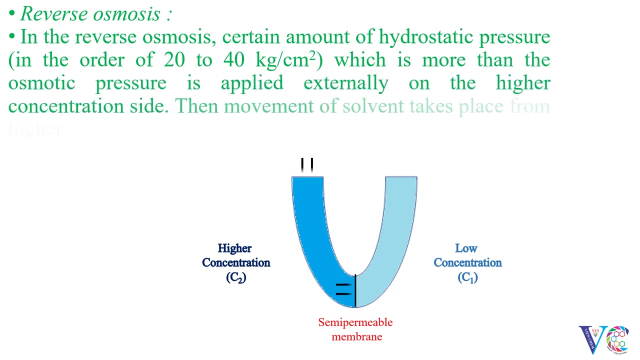 Reverse osmosis. In the reverse osmosis certain amount of hydrostatic pressure in the order of 20-40 kg per cm2,, which is more than the osmotic pressure, is applied externally on the higher concentration side. Then the movement of solvent takes place from higher concentration. 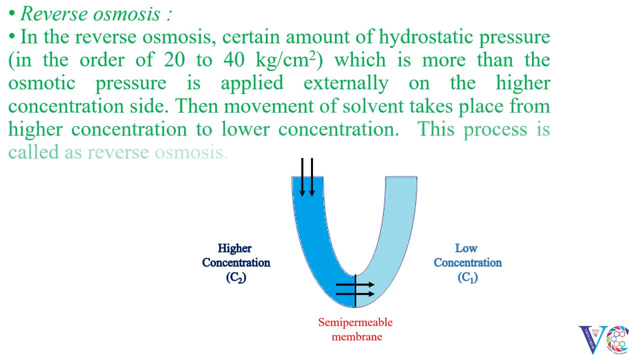 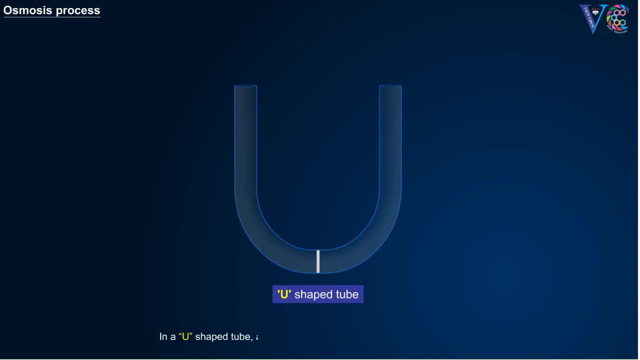 to lower concentration. This process is called as reverse osmosis- Osmosis In a U-shaped tube. a semi-permeable membrane is fitted at the center. One side: less concentrated solution- C1 is filled. On the other side, more concentrated solution- C2, is filled.